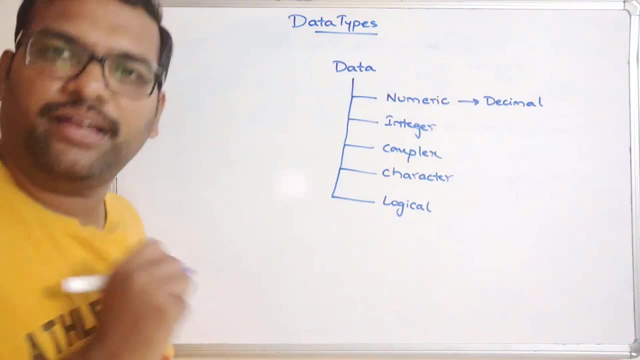 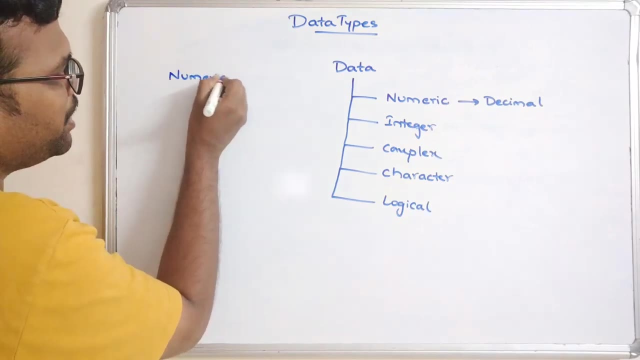 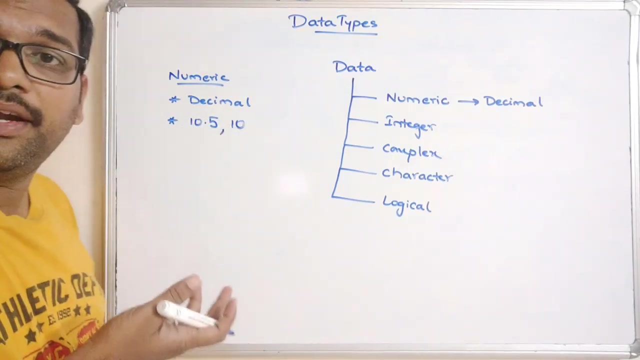 values comes in under this numeric data, including the whole numbers, right? So, for example, if it is a numeric data, so this is a decimal, and example, let us take some 10.5.. So that is a decimal value, and even 10, it is also a whole number, Everything. 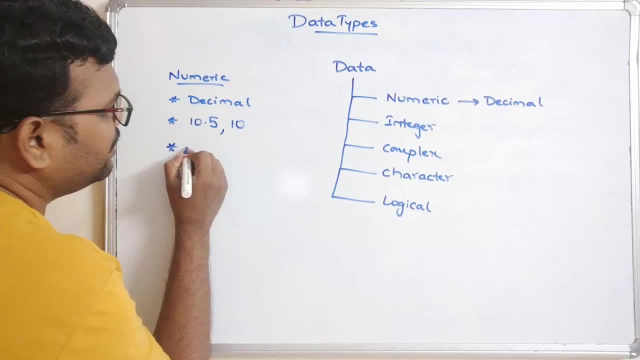 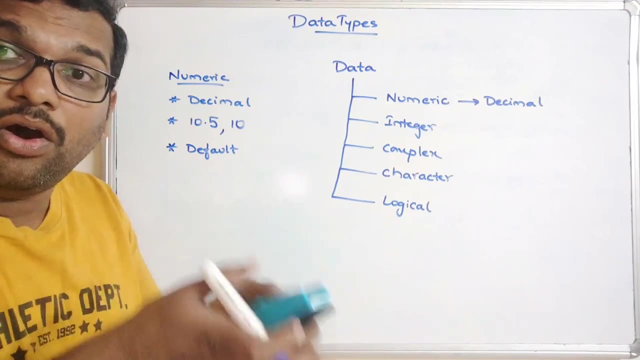 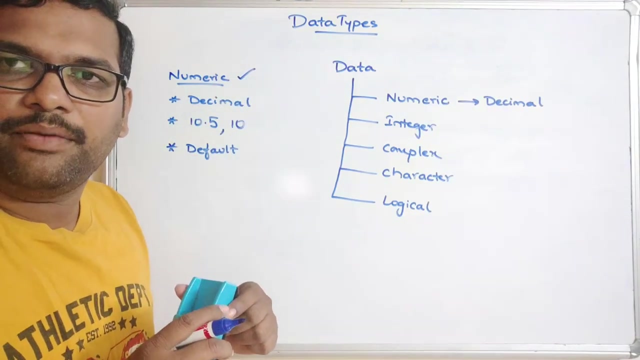 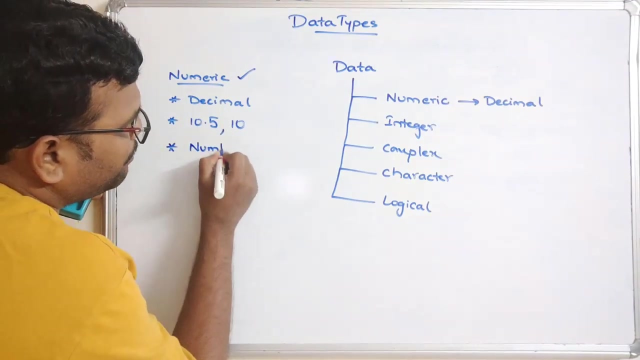 comes under the numeric and this is a default. I mean default means all the number data types. okay, All the numbered type is initially taken as a numeric data type. okay, See, not a default, we can say it as a number. okay, By default, if you assign any number to any variable. 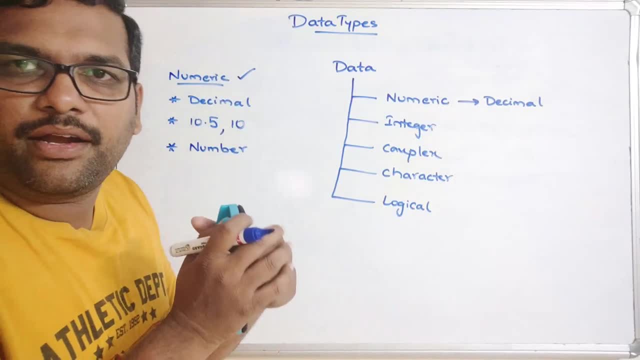 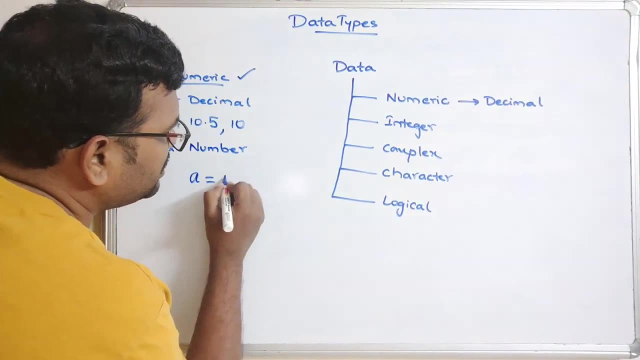 that will be defined as a numeric data type- numeric data type. So we know that assigning a value to a variable, some a, is equal to some 10. That is not a default. In fact, we now know it as a numeric. 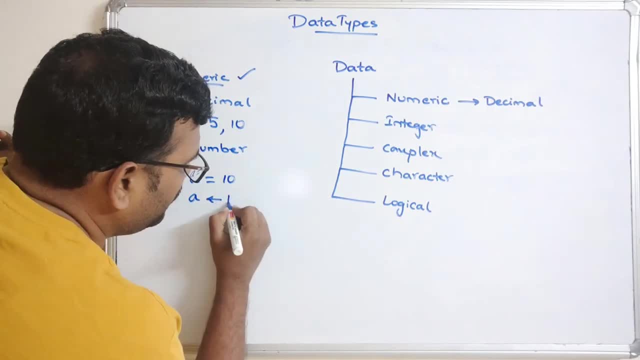 We know it has different type of data. We know it has property On third party with this particular value. we know it is 10, because we already know this prop hasential. if we assume that this is, then, then we will left word 10,. right, That means a is stored under. 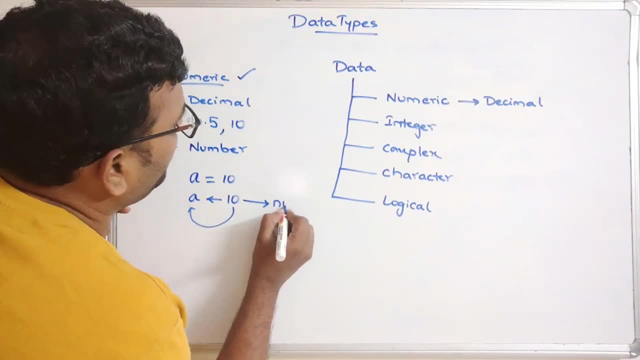 a name, a right. So here for a data type of a is numeric. numeric, For example, a is equal to 3.5.. Okay, or a is 3.5. So here also the data type is numeric. 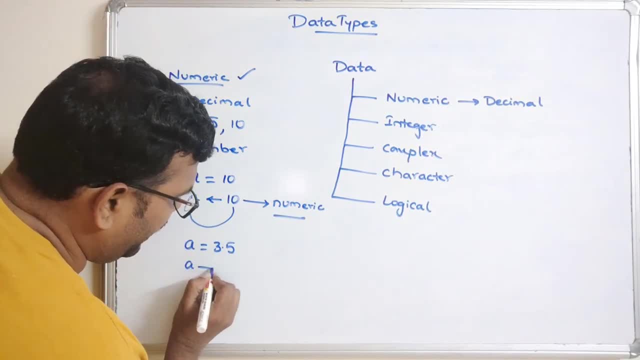 So by default, since Explained and made correct, We haveours clause form once right and Legato is all able to define. There are types inside that day. and when I talk about classical data on secondMar neurological data, we talk about ALECT, ORP or X0, right, Something like that. that 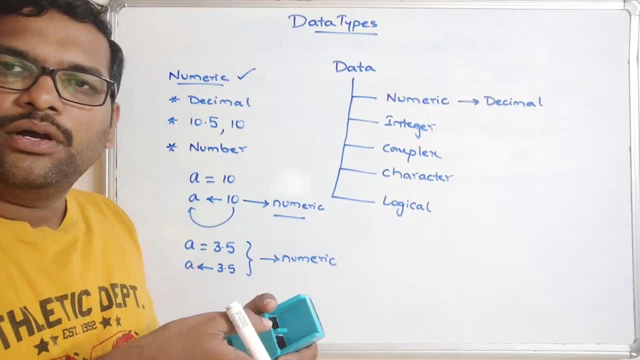 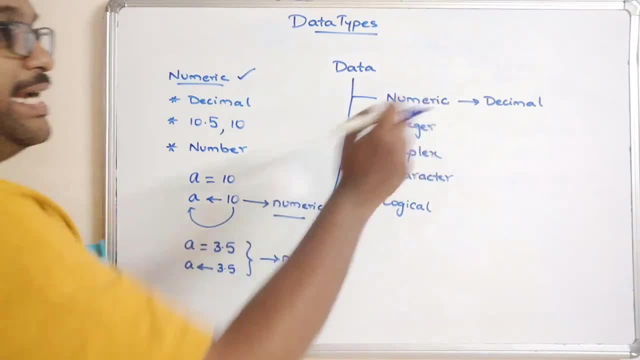 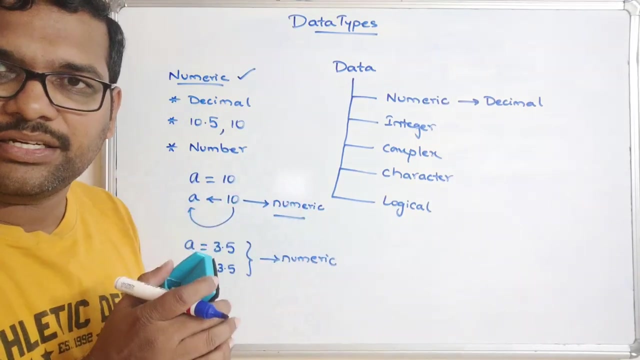 by default. if you assign any value- number value- to a variable, that will be considered as a numeric data pack, see. the next one is a integer. so we know that integers are only the whole numbers. so the decimal points will not be accepted in these integers, right? so how can we differentiate? 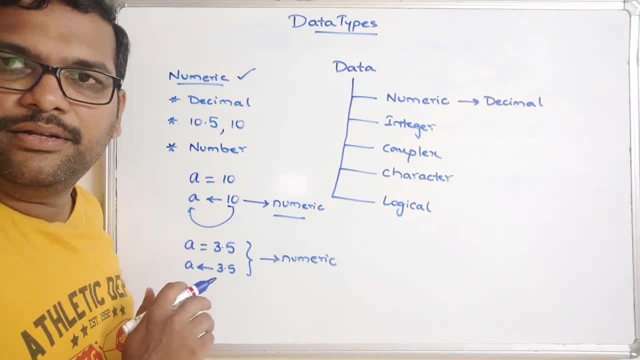 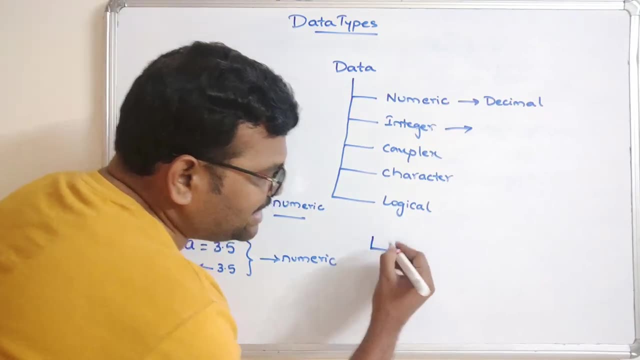 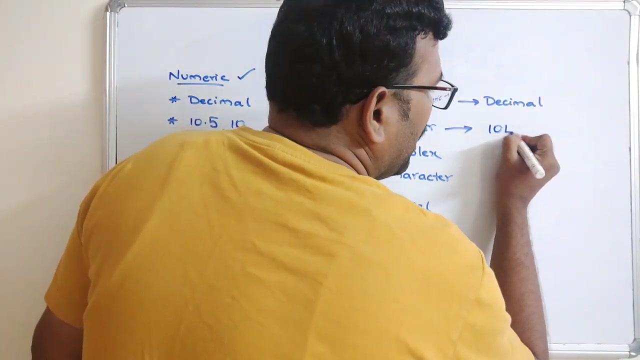 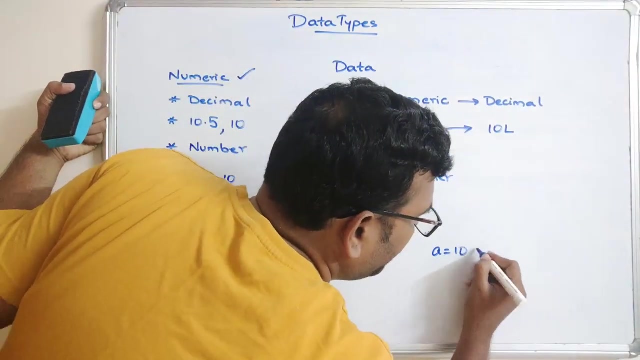 this 10 as a numeric or integer. so all the integers, all the integers will be having l as a end of a number which indicates the integer. for example, so 10 l, this is an integer data pack. so if you, if you are assigning some a is equal to 10, that will be a numeric that will 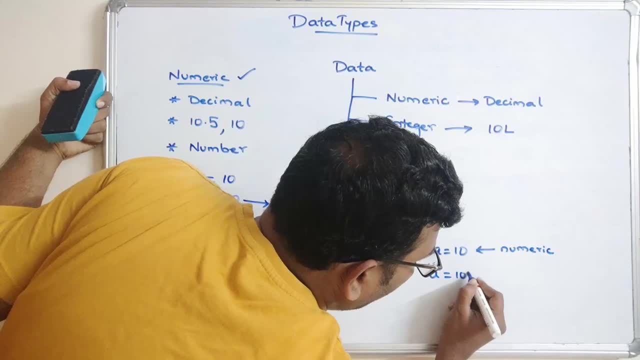 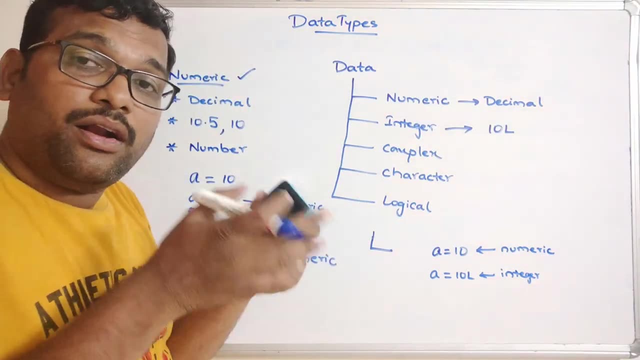 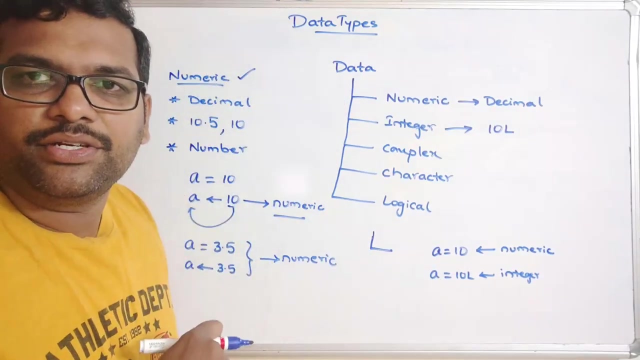 be a numeric data pack. if the same thing, a, is equal to 10, l, that will be integer data pack. so if you want to declare or store a variable, that will be a numeric data pack. so if you want to declare or store a variable as a integer, specifically, we have to use this l indication. so l is to represent the number is. 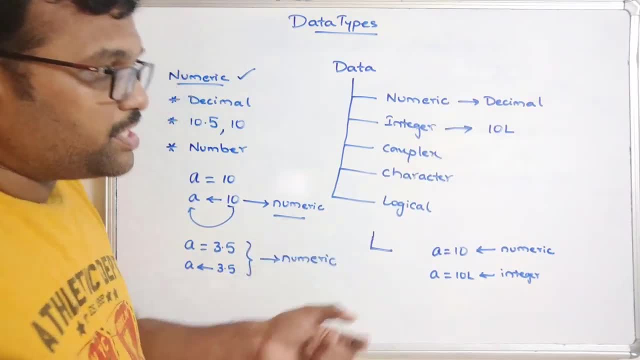 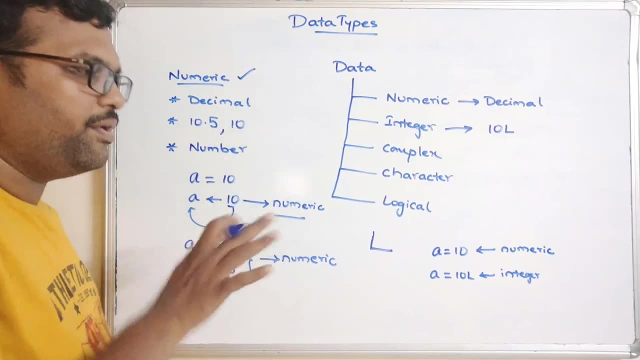 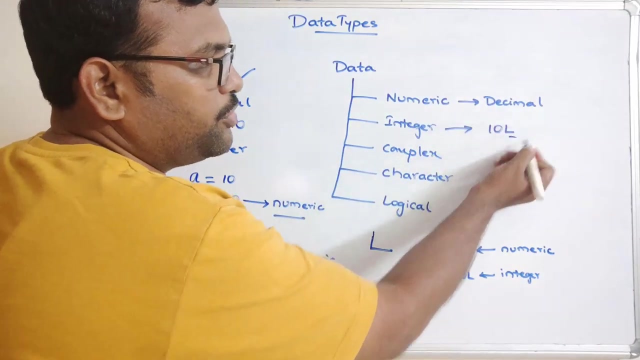 integer, right. so that is the main difference among this numeric and integer. so that's why i have said that if you assign any value, then by default the data type will be a numeric. if it is a number, right. so if you want to store the integer, just use a l, use a l, right. 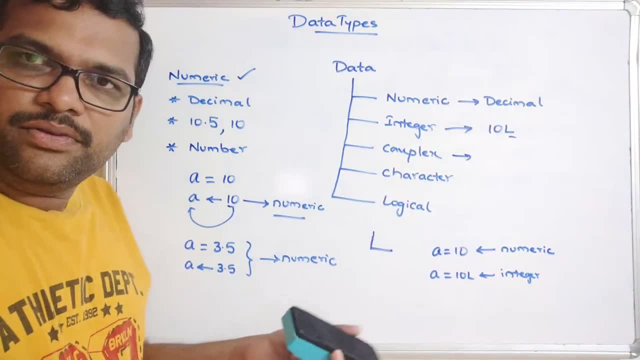 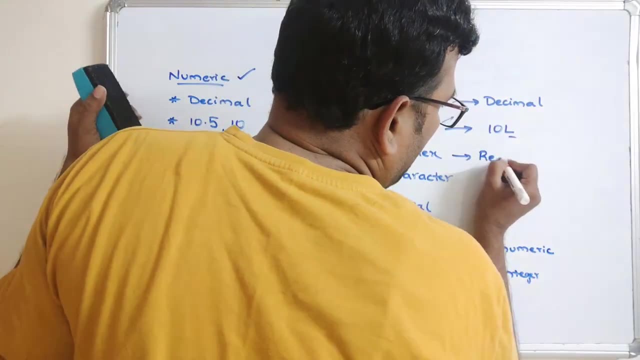 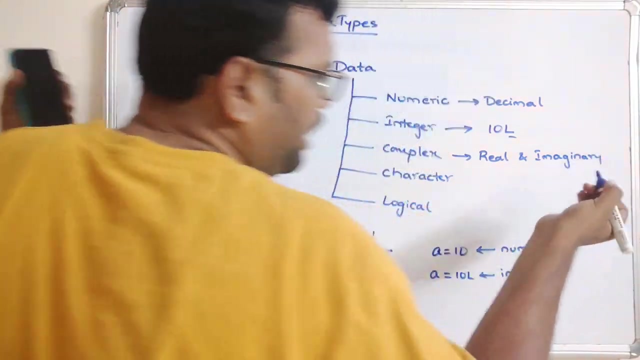 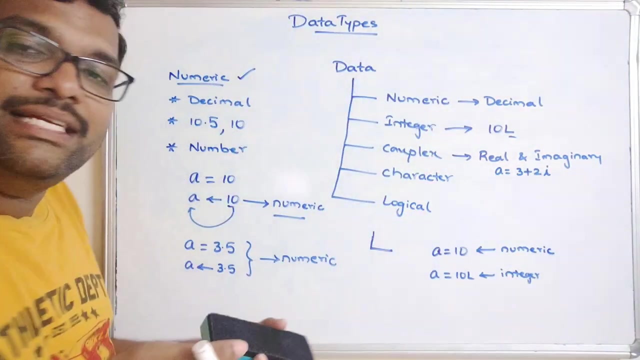 next, complex. so we know that a complex numbers, right, complex numbers are the numbers which are having the real part and the imaginary parts. right. so a real part and imaginary, imaginary. so example, we can say it as some: a is equal to 3 plus 2, i. so here i is nothing. 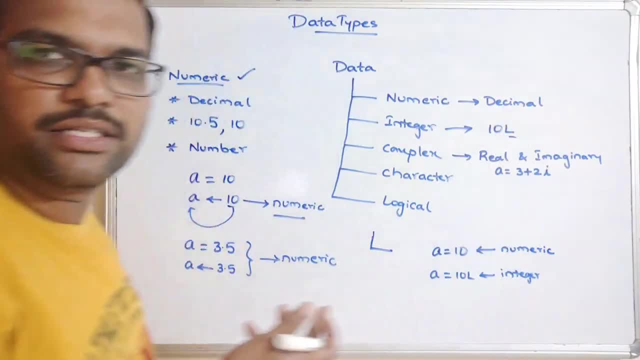 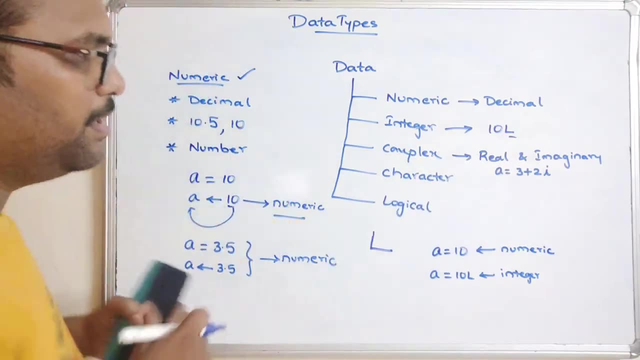 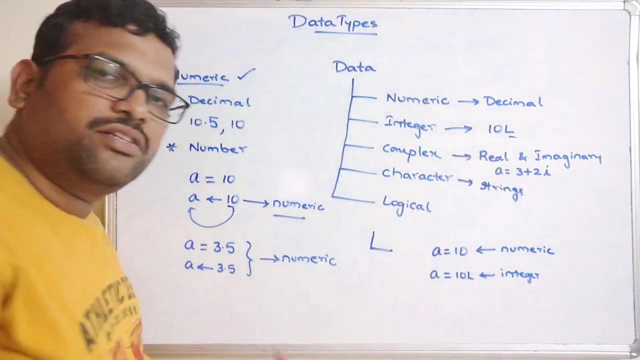 but an imaginary part, and a three is nothing but our real part. so these of numbers we call it as a complex, complex data type. complex data type. and the character: this is nothing but a strings, so group of characters or individual character, everything comes under this character data type, so strings. 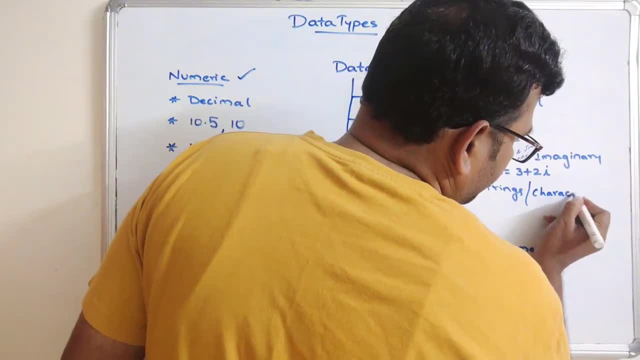 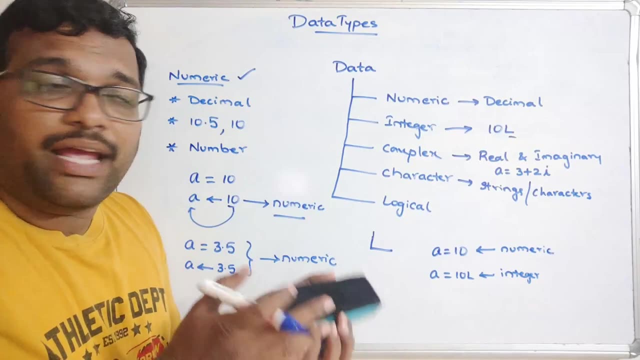 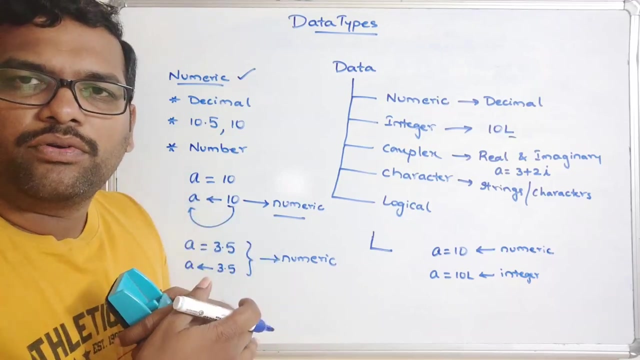 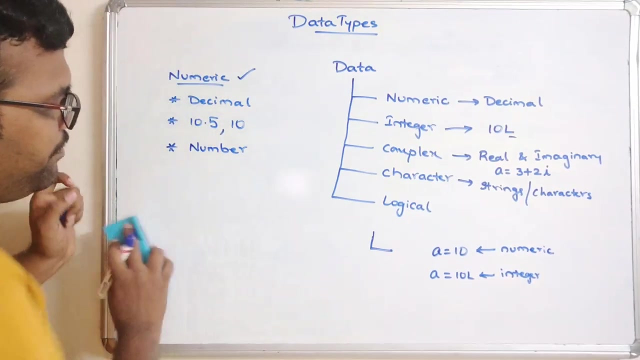 or characters, strings or characters, so which way, which we can call it as a strings, so actually the characters, a group of characters, we call it as a string. and what is the character? so every key in the keyboard can be considered as a characters. so we can consider, say, I'll write here characters. 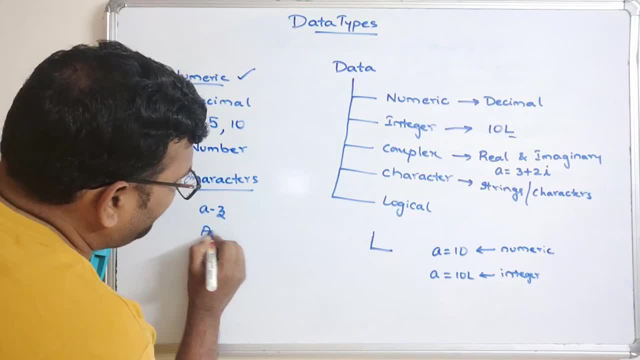 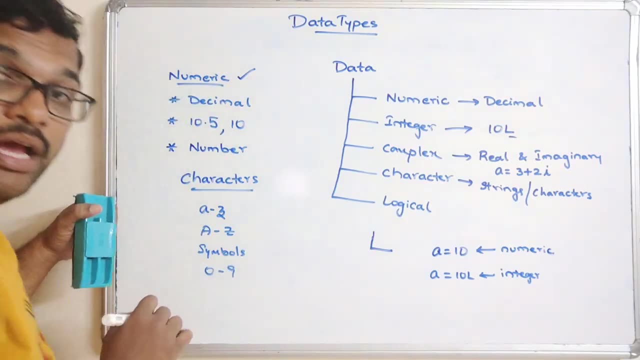 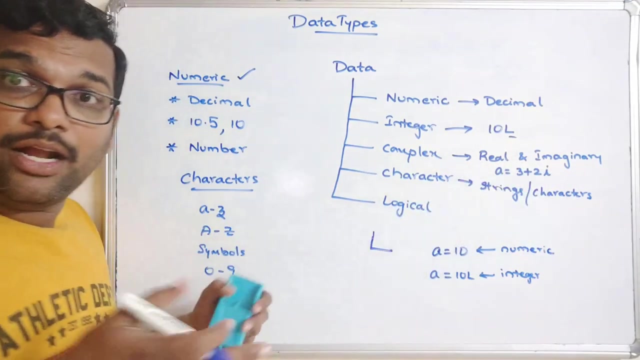 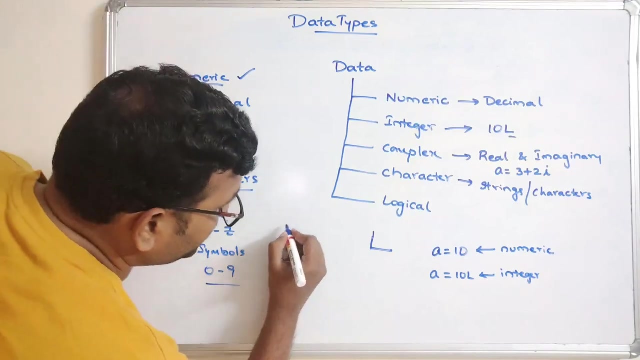 so a to z capital, E to capital J, symbols 0 to 9, okay, everything. so, whatever the key we have are observing in the keyboard, everything comes under this character and a group of characters. we call it as a string. so we are saying that 0 to 9 is also a string. so how can we differentiate? 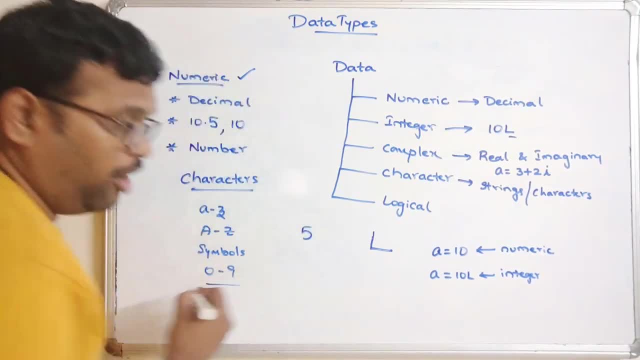 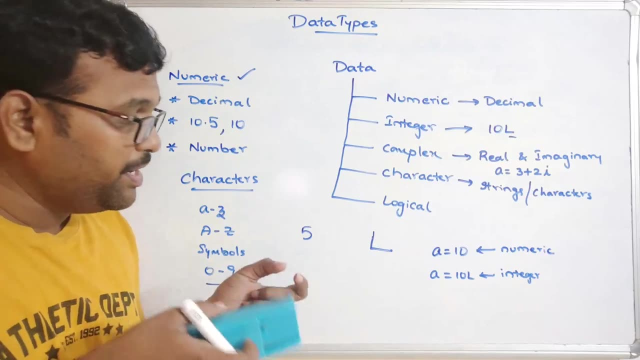 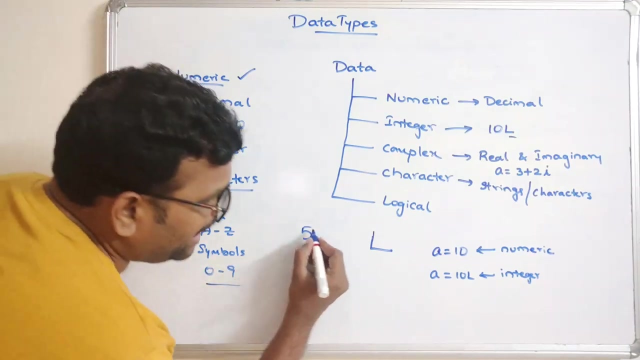 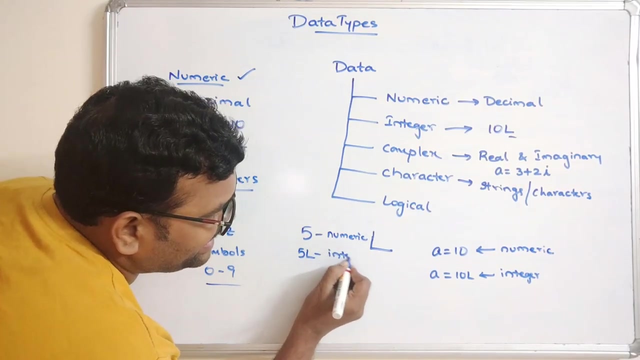 so if i, if i write as a 5, how can we know that the data type of this particular value, is it a string, or i mean, is it a character or integer or a numeric? so if it is 5, then it will be numeric, and if it is 5 l, it is integer, and if the 5 is enclosed in single quotations or 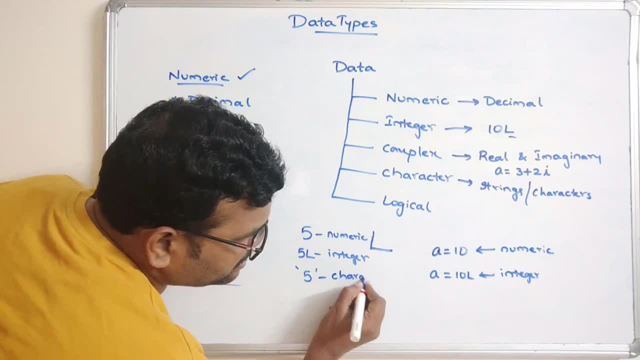 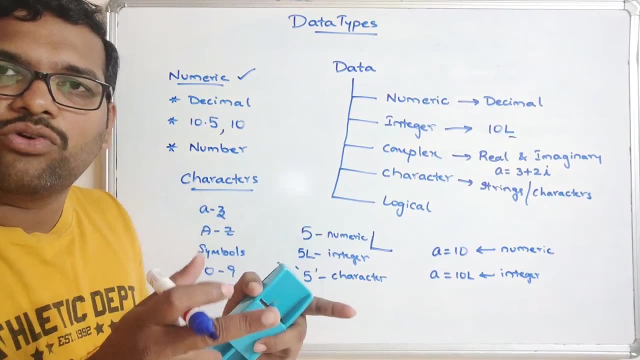 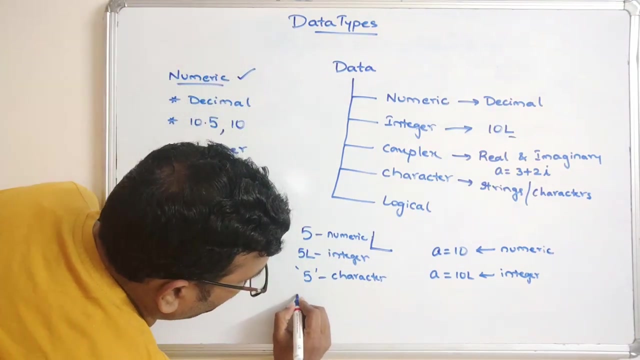 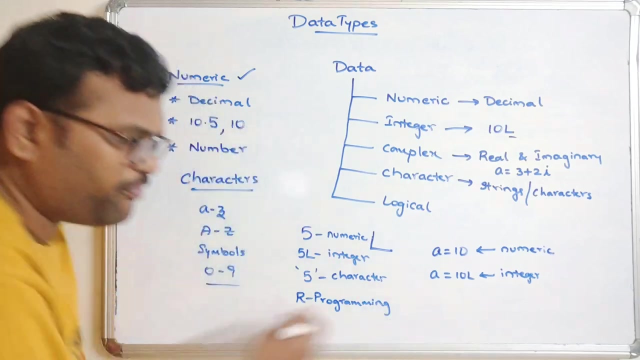 above quotations. that will come under character. all right, so every character must be enclosed in a single correlation quotation or a double quotations. so this is called a characters, for example random, are programming, are programming, so this is not even a group of characters. so we have seen symbols are also comes under the character. so here, 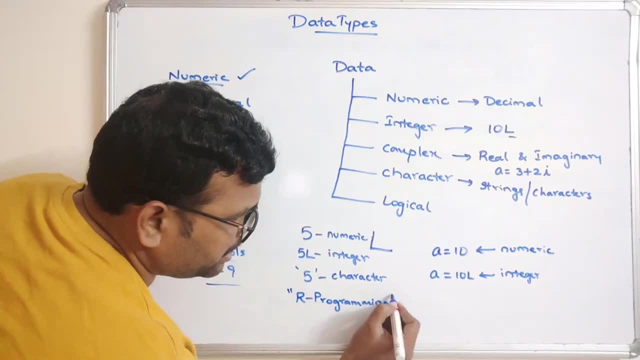 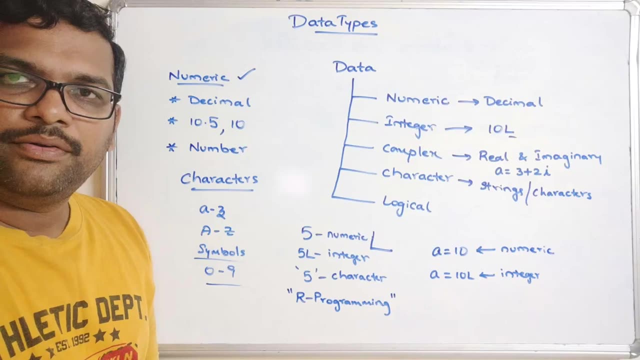 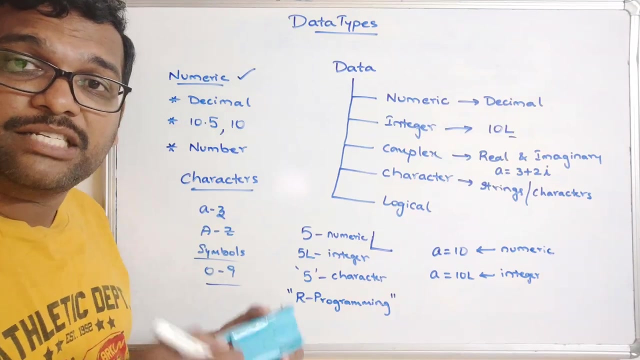 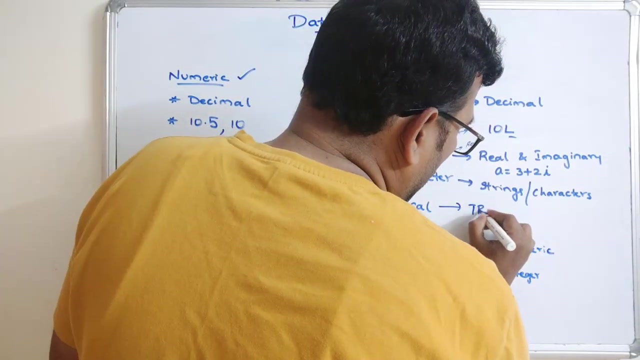 we are having some symbol, and this must be enclosing double quotations or a single quotations, then only this will be considered as a character data type. okay, character data type. so the last one is a logical. so logical data type is a special data type which will be having only two values, either true or false. so 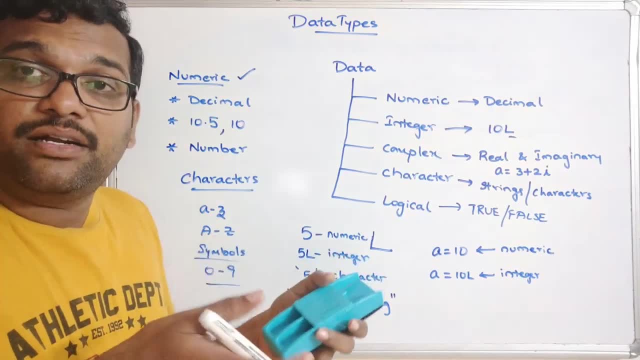 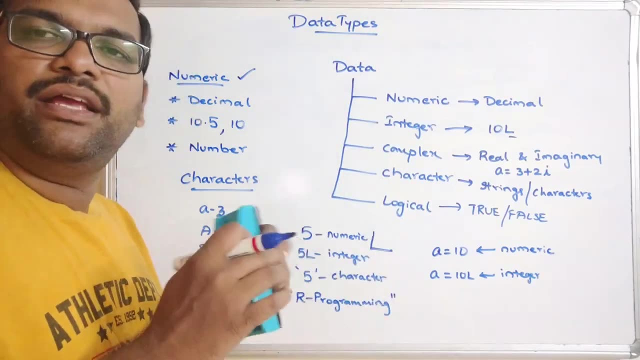 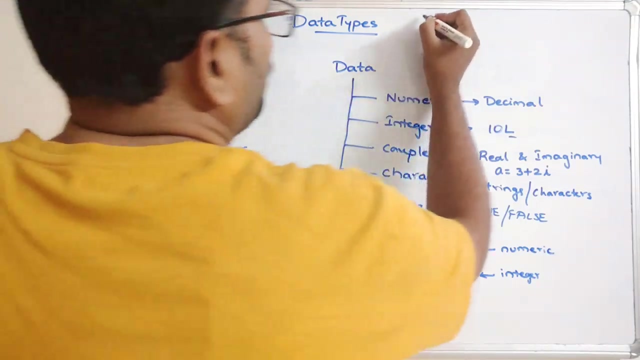 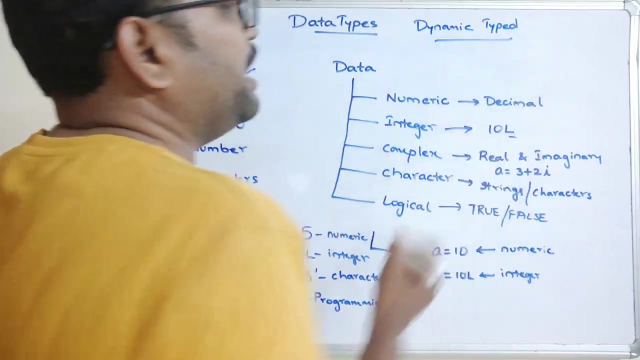 usually we call it as a boolean data type, right? so it will result only true or false, right? so these are the basic data types which are available in our world programming. and one more important point is our programming is a dynamically typed language. so dynamic typed language, dynamic type. so what is this dynamic? 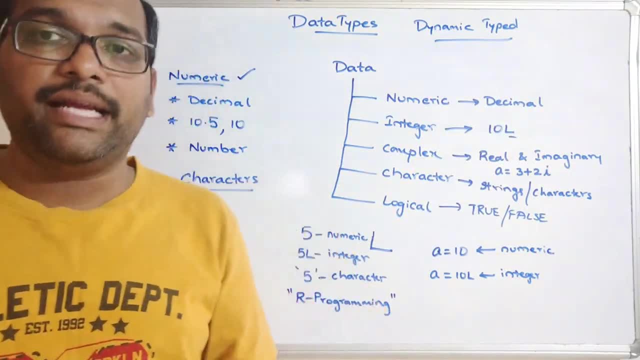 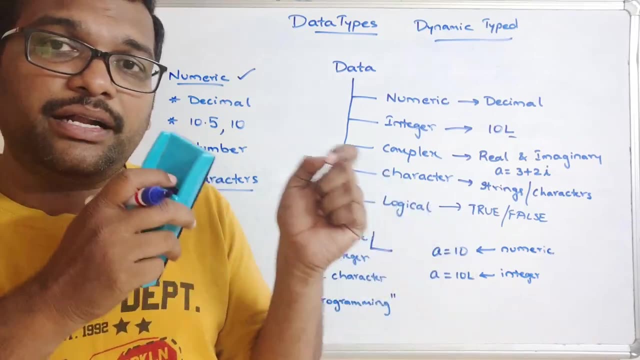 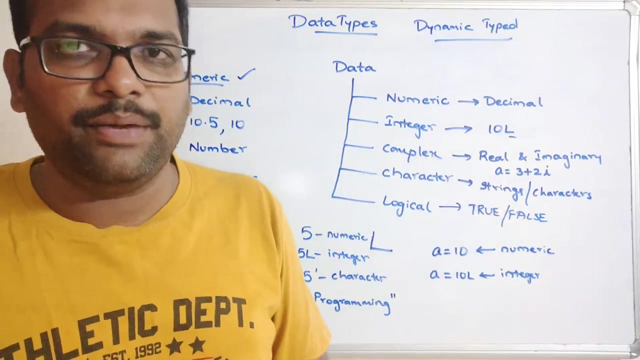 type. so dynamic type, it means we need not declare any variable explicitly, so directly we can assign a value to the variable and based upon the their type of value which we are assigning to a variable, the data type will be assigned to that particular variable. for example, if you consider here some a is equal to 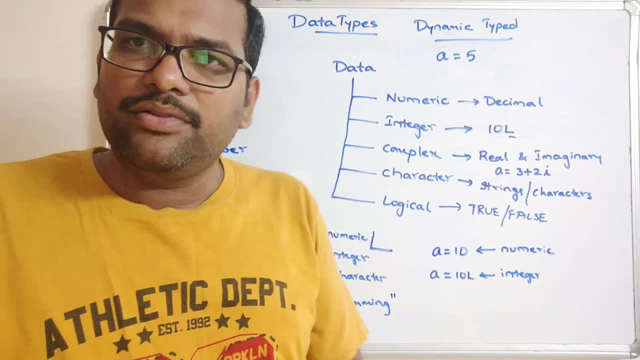 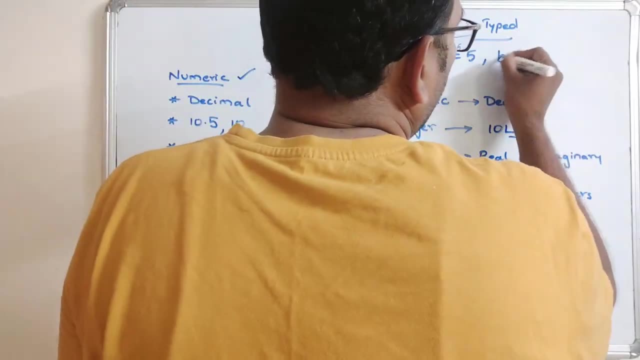 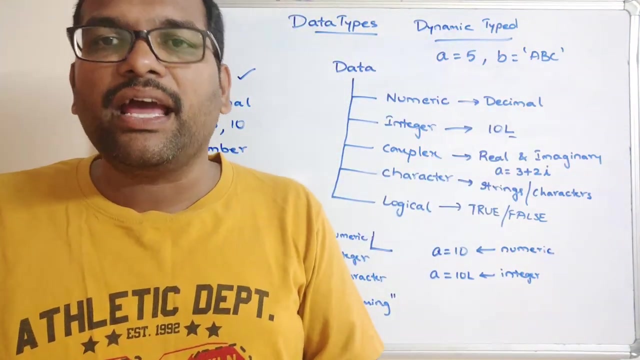 five. now what is the data type of a? so here the data type of a is a numeric data type, because five is a numeric data type, for example, if b is equal to abc, now the data type of b is a character data type, character data type because so. 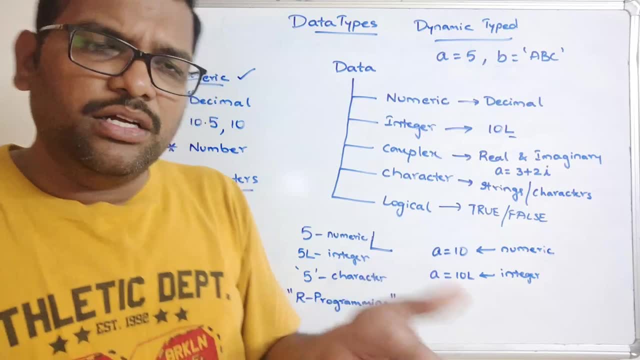 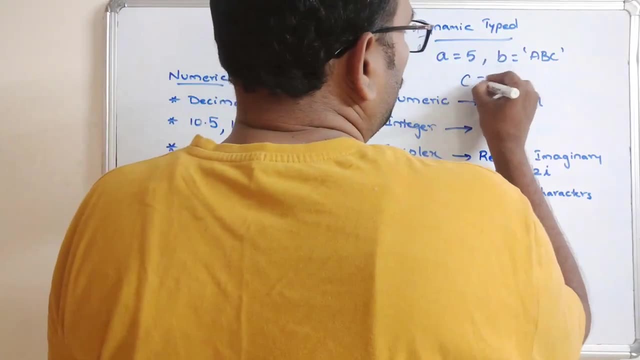 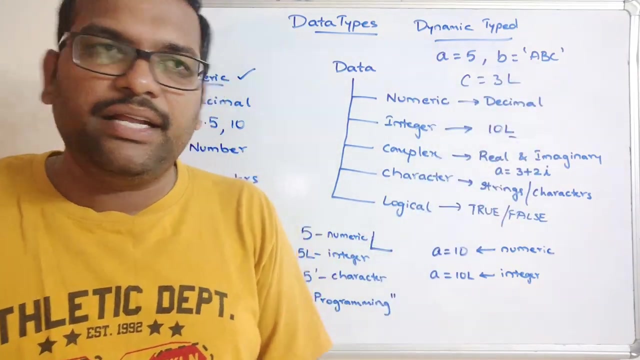 we are giving some group of characters enclosed in single quotations and the quotations, so you can enclosing single quotations for double quotations. okay, that doesn't issue. and similarly, some C is equal to 3 L, so obviously the number ends with L, which indicates the integer. so C will be the integer data type. now. 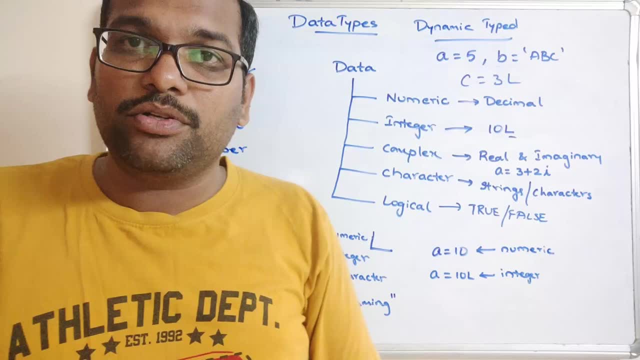 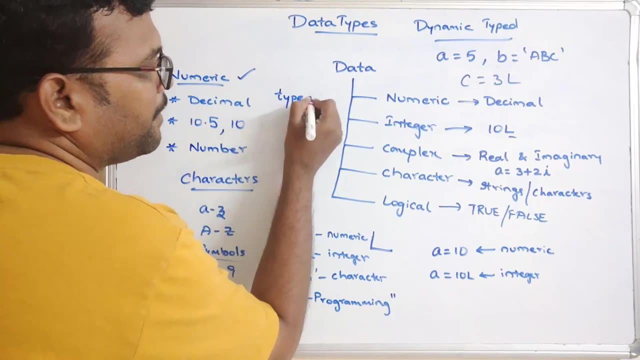 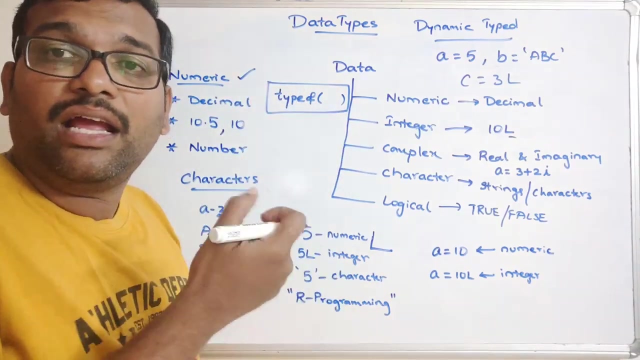 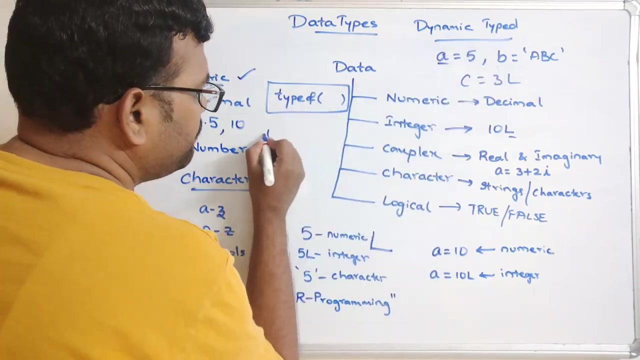 how can we know the data type of that particular variable? so in our programming we are having a function called typeof, typeof. so this type of function will give the data type of a particular variable which pass to this particular function. if you want to know the data type of A, simply you can give. 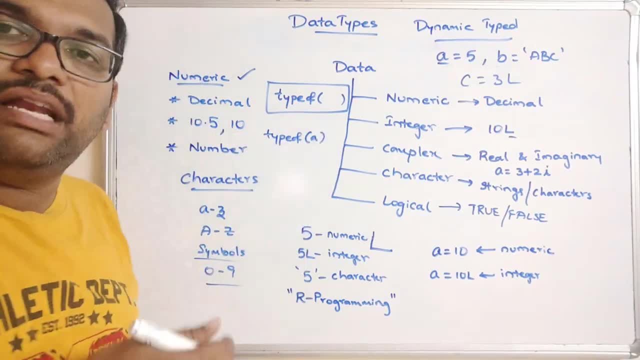 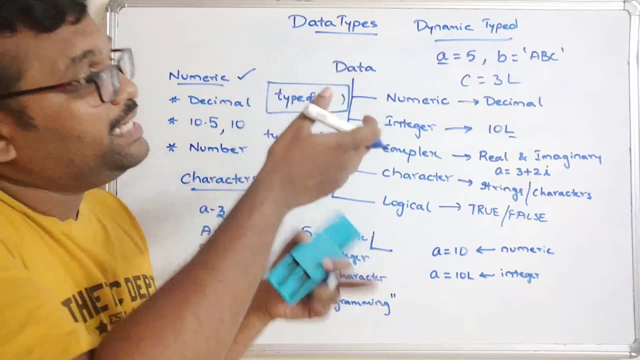 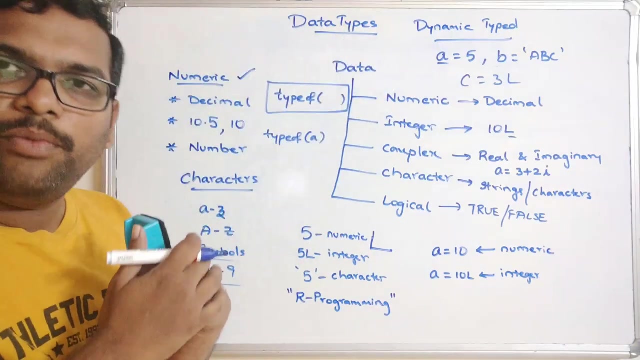 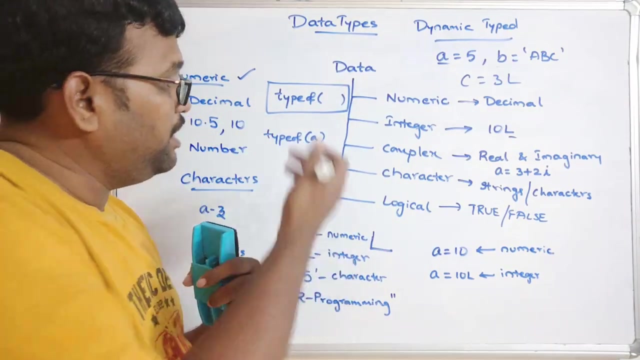 typeof A automatically will return the data type of this particular variable. and one more important thing: so we will call. call all these as an objects. So the data type of object A will be a numeric data type and object. the data type of object B will be a character data type and similarly the data type of object C. 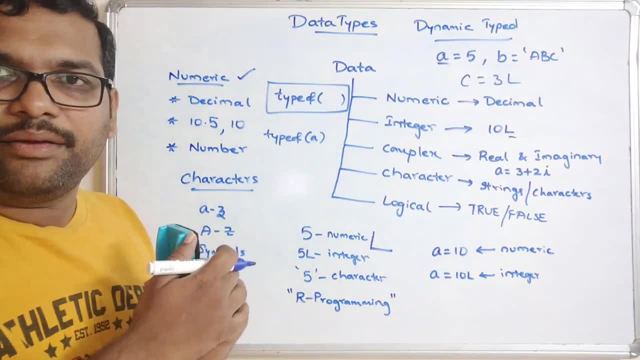 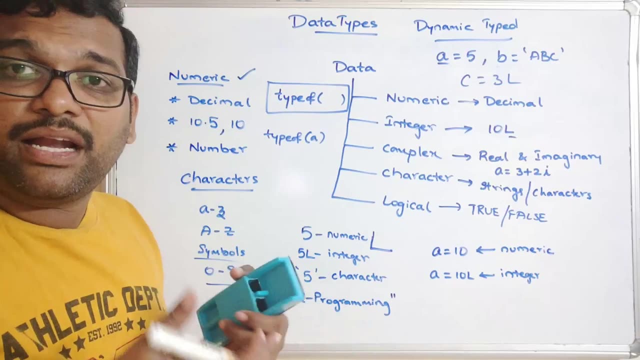 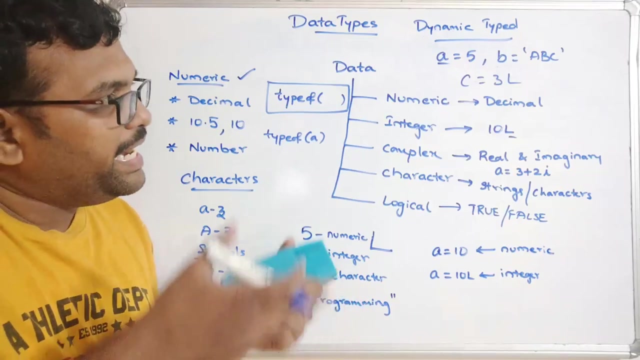 will be the integer data type, So like that. so we need not declare the variable with a specific data type explicitly. So we are not declaring any variable. So based upon the value assigned to that particular variable, the data type will be defined there. So such type of thing we call. 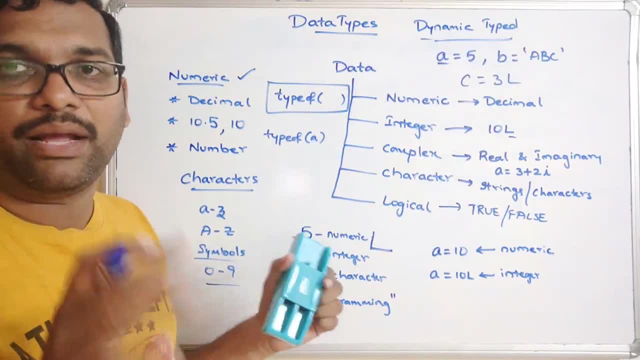 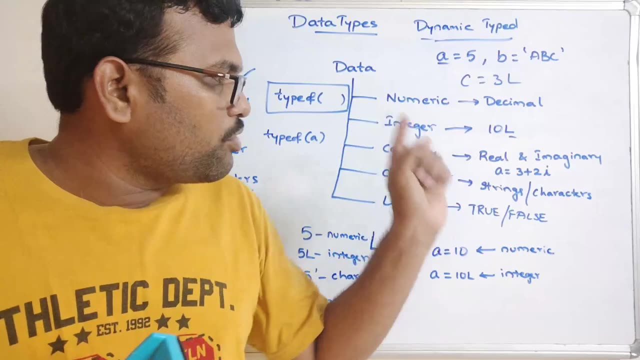 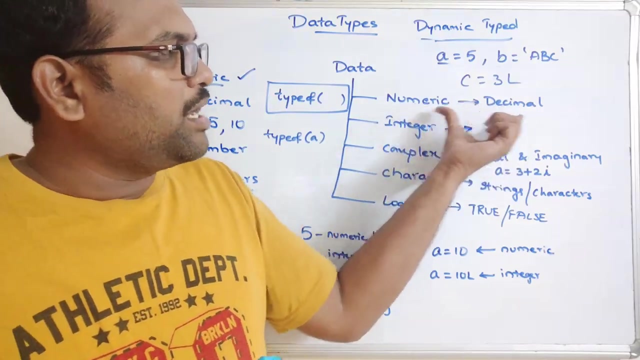 it as a dynamic type of language. dynamic type of language, right. So hope you understood the basic data types available in R programming. So numeric, integer, complex character and logical. and there is a slight difference among this numeric and integer. So see, the numeric comes with a decimal. 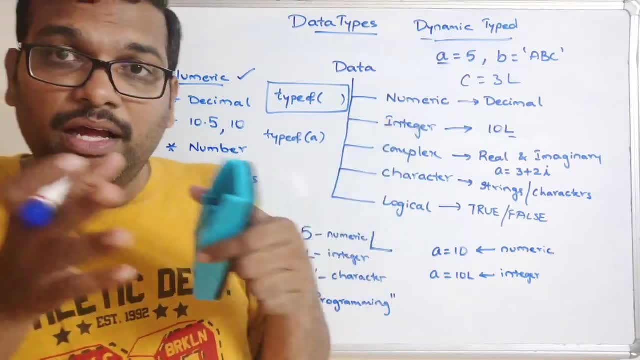 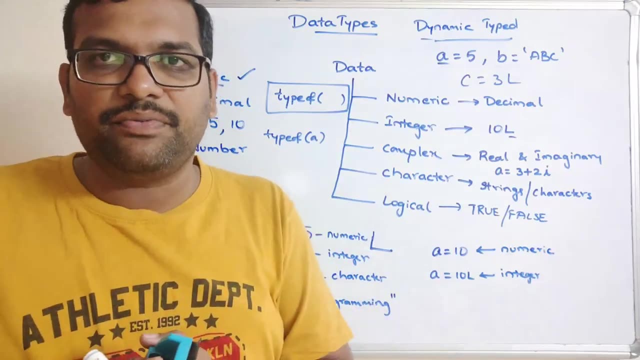 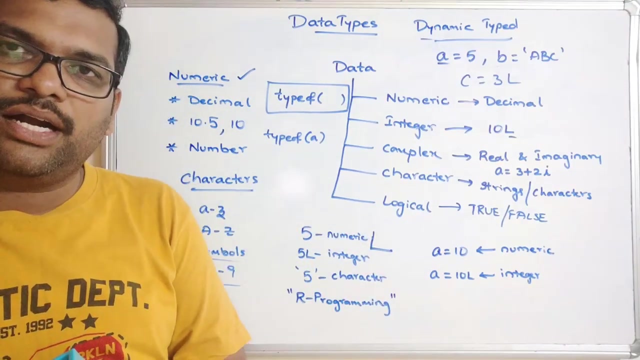 value As well as the whole numbers, and integer comes with the only whole numbers with L, specifying with L. L indicates the integer value, right? So hope you understood this one. Let us stop here and if you are, if you are having any doubts regarding this concept, feel free to post your 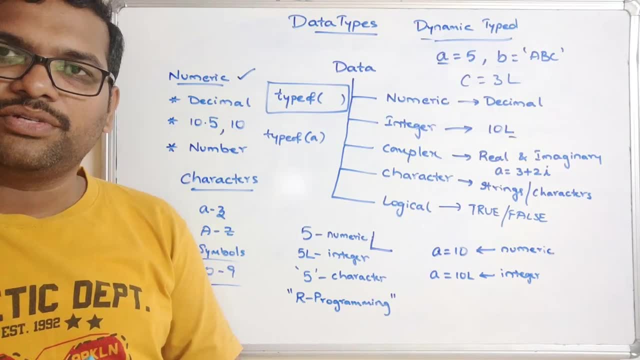 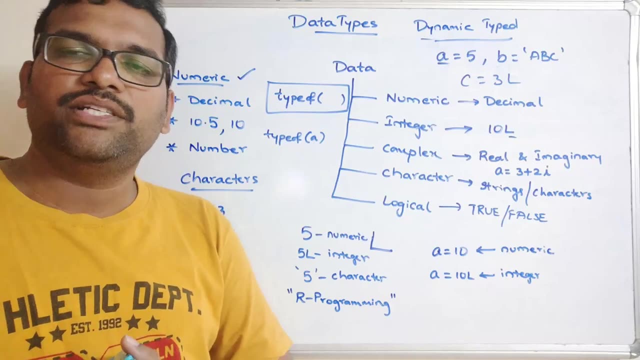 doubts in the comment section. Definitely, I will try to clarify all your doubts and if you really enjoyed my session, like my session, share my session with your friends and don't forget to subscribe to our channel. Thanks for watching. Thank you very much.